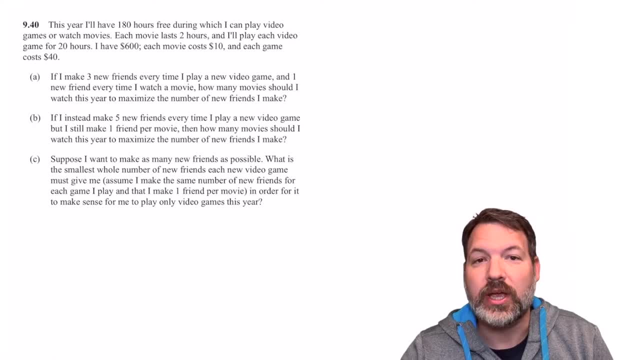 six hundred dollars. each movie costs ten dollars and each game costs forty dollars. What I typically recommend is that we want to begin by asking ourselves, on these kinds of problems, what are the constraints, That is, what are my limited resources that are going to help? 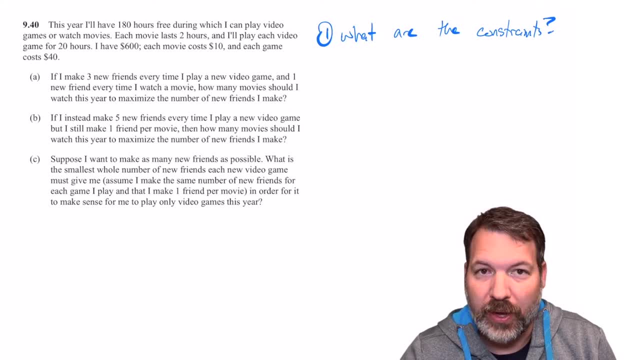 determine how much time I spend on blank, whatever it might be. In this particular case, you can tell there are two limited resources. There's the time I have to actually watch the movies and play the video games, and then there is the money I have to spend on the movies and the video games. In both, 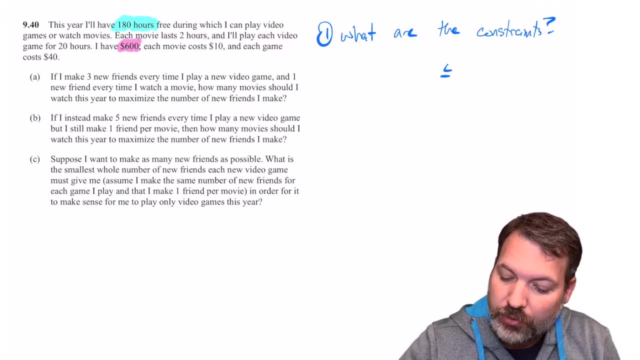 cases these are less than or equal to constraints. I have a limited amount of time to spend on the movies. I have up to 180 hours. I have up to six hundred dollars to spend. So those are our two constraints. We'll even jot down, just so we remember for the future, this first constraint. 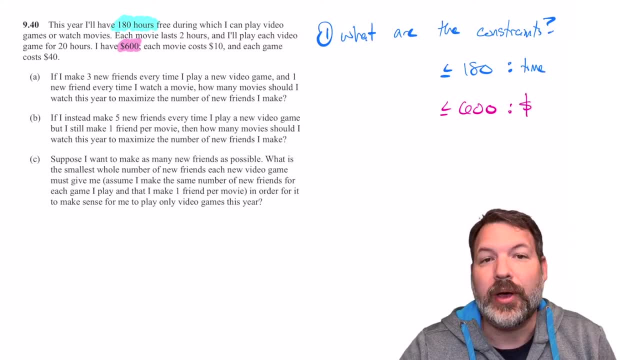 is about time. This second constraint is about money. From there, we want to ask ourselves: what do we not know? The answer to this question is going to be our unknowns. It's what we're going to use to assign variables. So we're going to assign variables In this particular case. 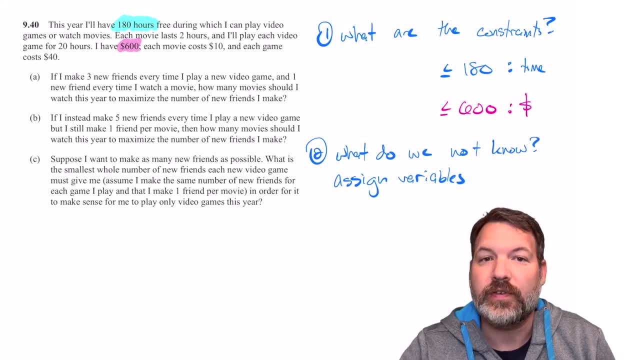 the unknown is: how many movies do we watch, How many video games do we purchase? And so we're just going to say: x equals the number of movies that we watch this year, and y will be the number of video games. That's also not the number of video games. We want variables so that we can go. 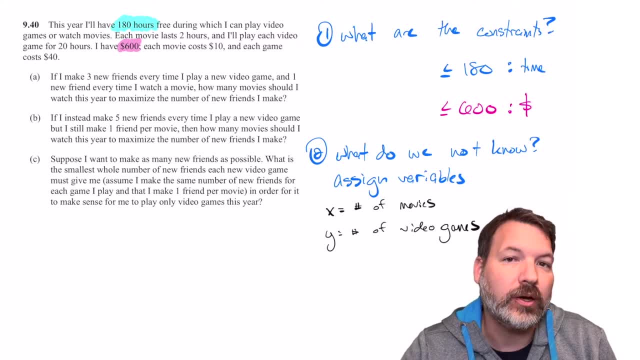 back to these constraints and write some linear inequalities, Linear in two variables, x and y, and we're going to graph these on a coordinate basis. For example, let's think about our time inequality. We know that each movie lasts two hours. Now we don't know how many there are. That's why we assigned that a variable. But 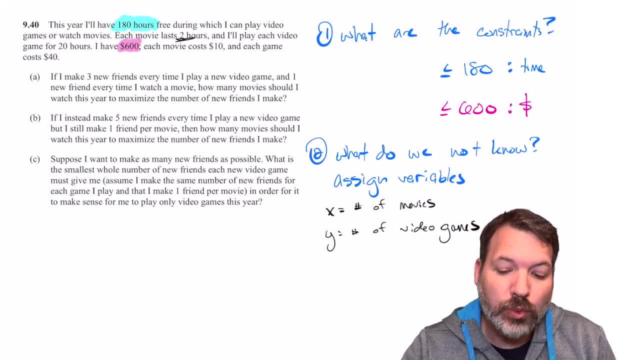 imagine that we chose to watch five movies this year. If each one of them is two hours, five times two makes ten hours devoted to watching movies. If I watch ten movies instead, it's going to take twenty hours. But what's important to recognize is, in each case: 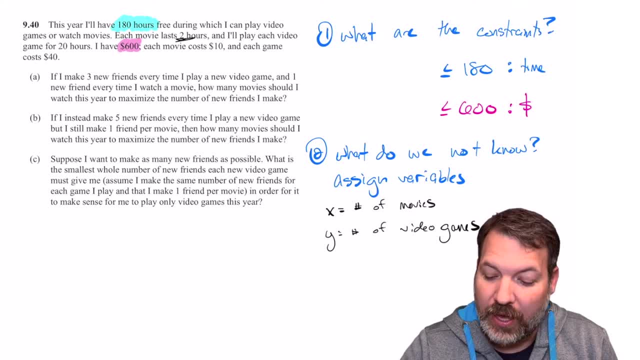 I'm taking. whatever that number of movies is- five, ten or our unknown x- and multiplying it with the number of movies that I'm watching this year, and multiplying it with the number of movies that I'm watching this year and multiplying it with the number of movies that I'm watching this. 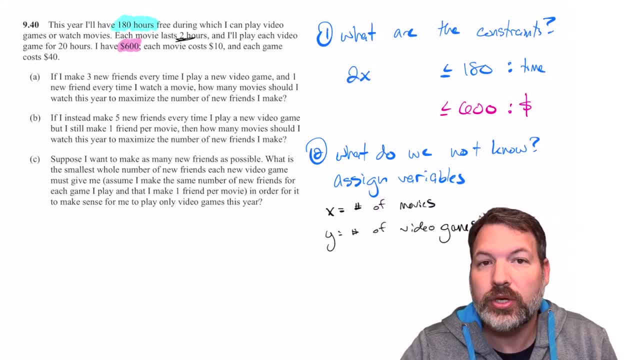 year and multiplying it by two, And so that's what's going to show up in the inequality. Two x accounts for the number of hours that I spend on movies. Twenty y is what's going to account for the amount of time I spend on video games. So we end up with this linear inequality. 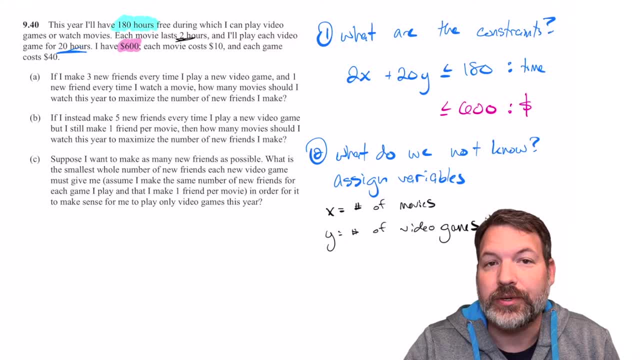 Two x plus twenty y is less than or equal to a hundred and eighty. We're going to do the same thing for the money. We're looking for some kinds of numbers in the problem that we can use as weights or coefficients. In this case, you can see, each movie costs ten dollars, and so in our 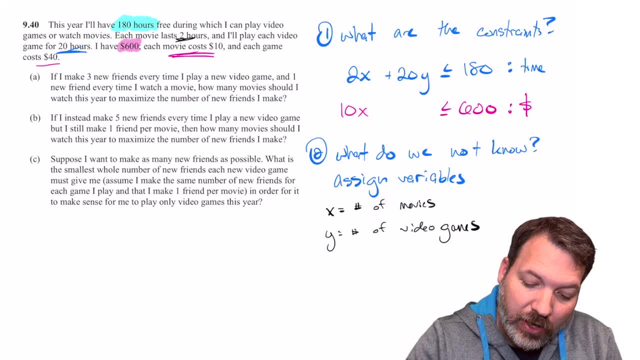 inequality. that's going to show up as ten x. and each video game costs forty dollars, So that's going to show up as forty y. And there's our second inequality: Ten x plus forty y has to be less than or equal to six hundred. That is, the ten dollars per movie times the x number of movies. 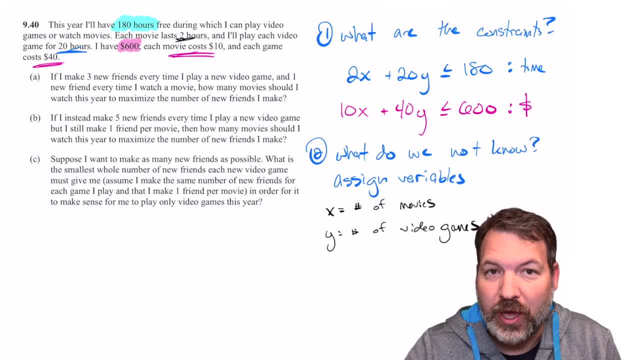 plus the forty dollars per video game times, the number of video games is going to be less than, or equal to, the six hundred dollars that I have to spend Now. probably the best thing to do at this point would be to utilize some kind of graphing calculator to graph these two inequalities and figure out the points that we need to know. 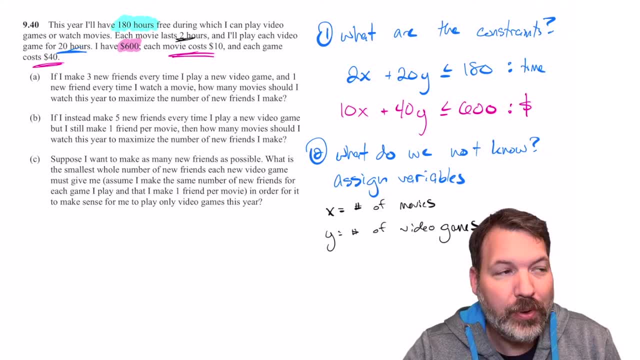 all of which represent possible solutions in this problem. But before we go to the calculator- we are going to use Desmos here in a second to do this- Before we go to the calculator, I just want to think through broad strokes. What are the kind of most extreme possibilities? 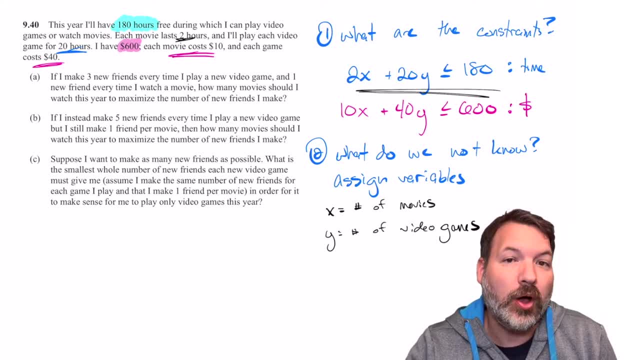 Concentrate on just one inequality at a time. Let's think about only the time that we have to spend watching movies and playing video games for a second. If I spend all 180 of my hours just on movies, that is basically if I ignore the video games entirely. 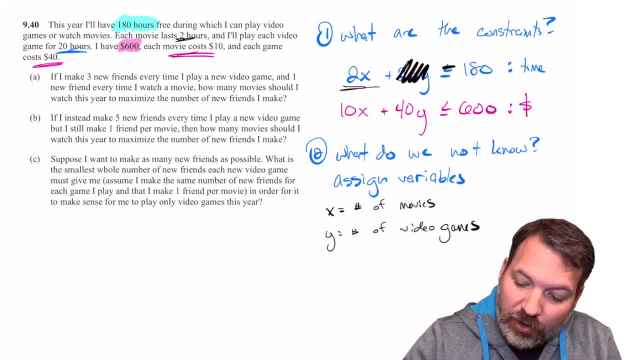 how many movies could I watch? Well, you can tell. first of all, let's say that this is equal to rather than less than because we want to use all 180 hours. two hours per movie times what number makes 180.. We can just divide 180 by 2 to figure out that that number is 90.. This corresponds to: 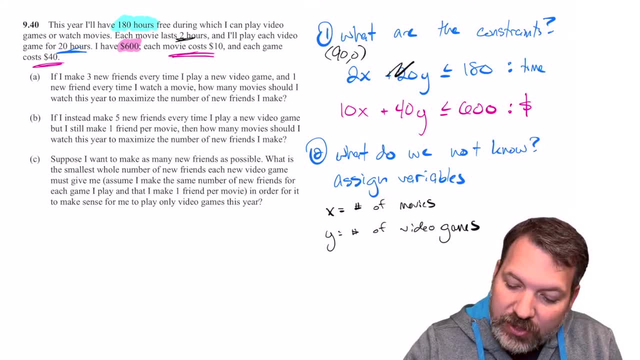 the x-intercept of that first inequality. If I assume no time at all on the video games but all my time on movies, I could watch 90 movies given the 180 total hours that are available to me. Similarly, if I went the other direction and said 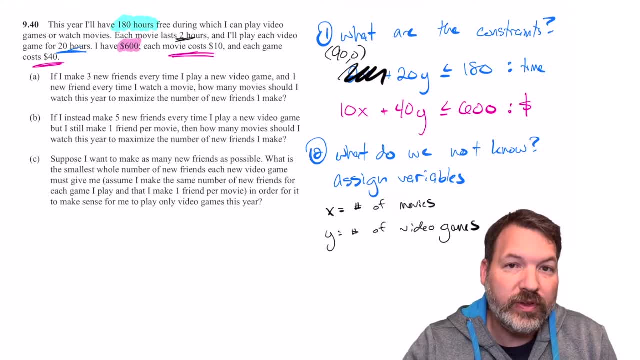 let's only play video games this year. that would mean that my movies are 0 and I can solve for video games. 20y equals 180.. Once again, we divide by that coefficient of 20 and we get that we could play 9 video games. So we're going to put that down here as our y-intercept – 0,9.. 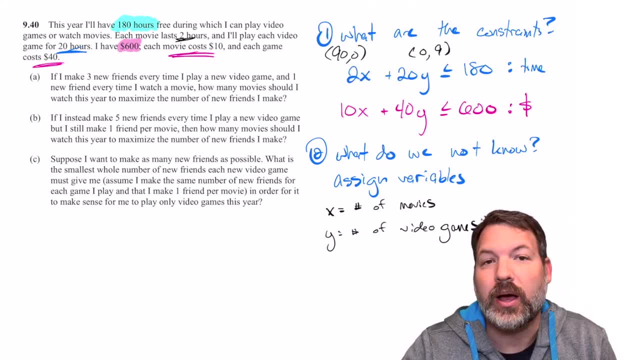 This will also be the first fisheryDamon bore, so the next contribution I'm going to give is for those of you who have not made the obvious guess about the answer aright, and most parole-eko about this 0,9.. The purpose of this isn't necessarily just to get it down on a graph Again, we can have a. 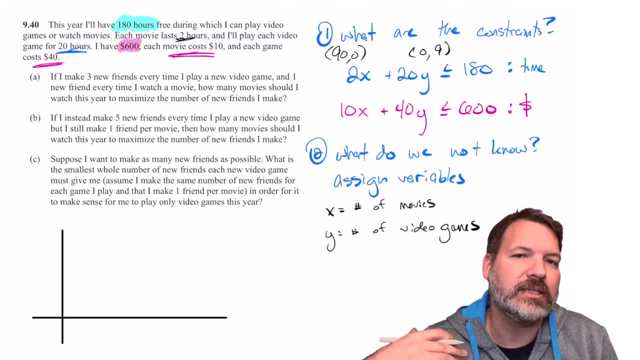 graphing utility do that part for us. The purpose is to get some intuition for what the possible solutions look like In this case. maybe we'll put 90,0 way over here. Let's just say that that's 90,0 and 0,9.. Maybe that's a little bit too high. 0,9 we'll put somewhere up here on our y-axis. 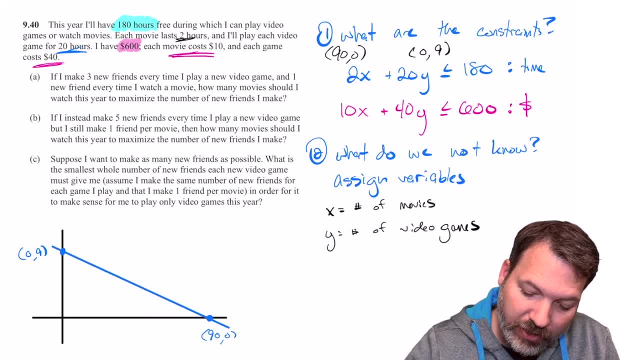 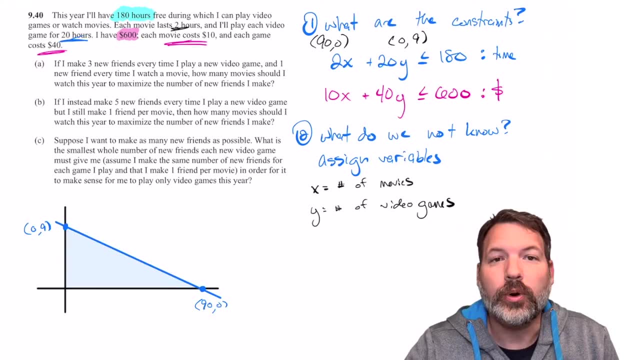 Our first inequality is going to be the solution space below this line, That is, we're interested in all the positive values. I need to move that around a little bit. We're interested in the solution space underneath this line because we could use up to those 180 total hours The line. 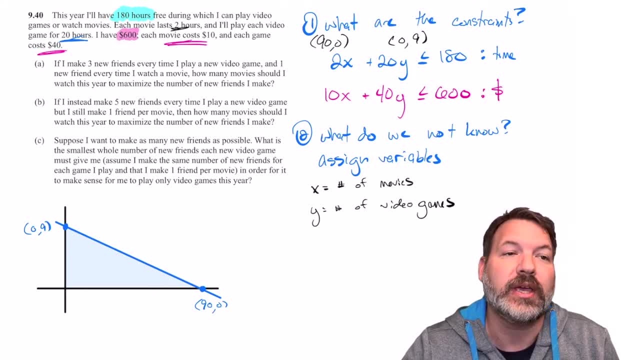 our boundary represents different possible solutions. if we use exactly 180 hours, Let's do exactly the same thing with our second inequality Again, if we completely ignore the video games and we only spend money on movies- $10 per movie for 600 total dollars- divide by 10,, divide by 10, we get 60,0.. We could watch 60. 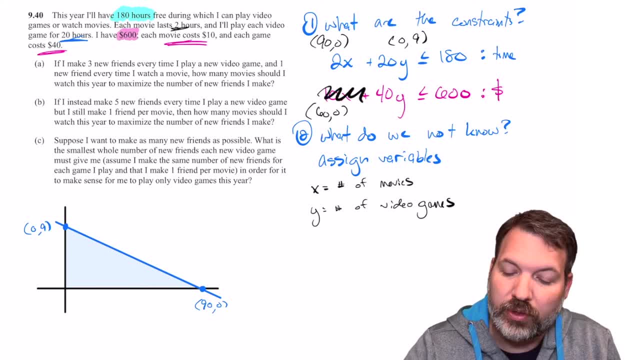 movies this year. just with respect to money. Similarly, ignore the movies for a moment. If each video game costs $40, and again we have our $600 to spend, divide by 40,, divide by 40, and that gives us 0,15.. If we only purchased video games, we could buy 15 of them. 0,15 would. 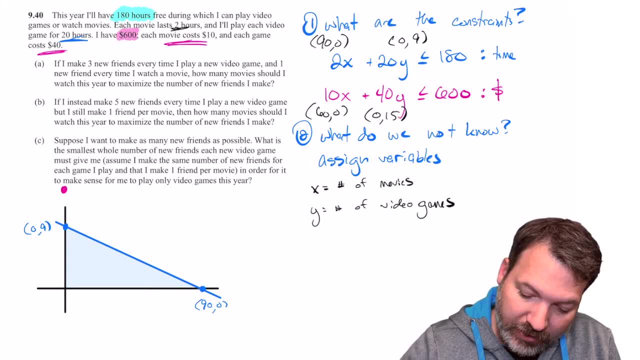 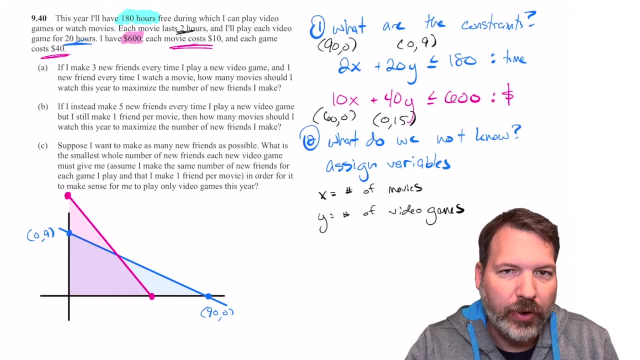 be somewhere up here, higher than our previous inequality, If we only purchased video games $100 per movie for 500 total hours. Again, we're interested in the solution space underneath below that line. Now, this is a very typical picture for these linear programming questions. 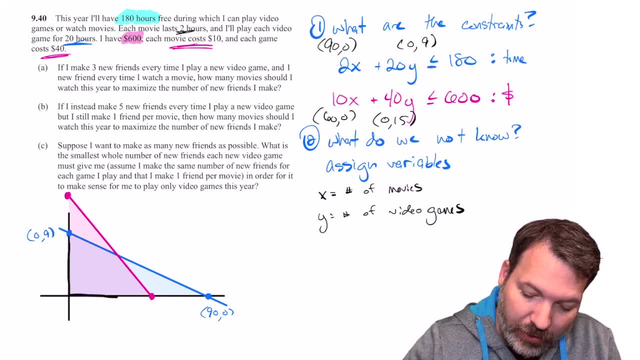 If we have just two constraints. this kind of diamond shape here is going to be something we see very often, and several of these corners we already know. Now, the reason I'm specifically mentioning the corners is- and here's the biggest- if we're going to be able to see the 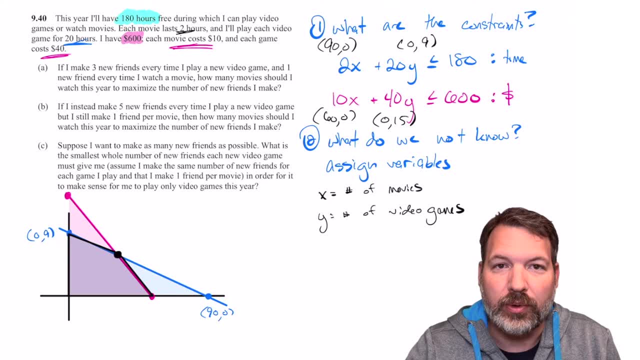 bottom of the screen. we're going to want to have a little bit of dimension in between beauty of this process. the solution to linear programming problems must be at one of the corners of the region When we take this to Desmos. in a second I'll show you precisely why that is. 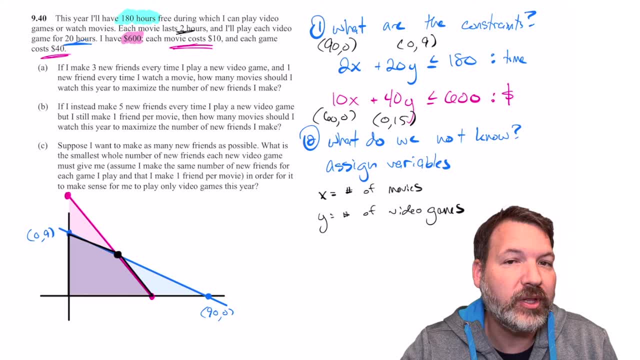 but for now, just know, all we care about are the corners. Our only possible optimizing solutions have to be at these corners. So right now we have several candidates for possible solutions to this problem. We've got 0,9.. That is this kind of upper left-hand corner here. We've got. 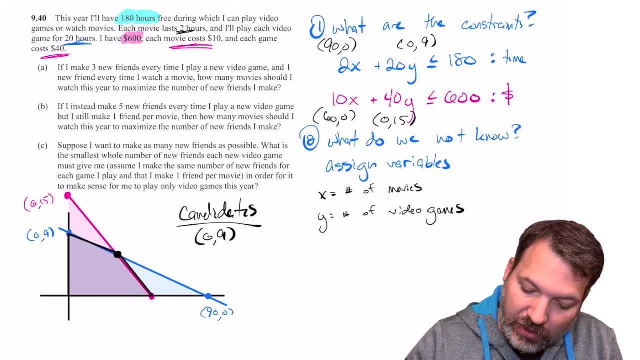 oh, I forgot to write these down. So this is 0,15.. This is 60,0.. And so we've got 60,0 as another possible candidate for our maximizing point. We also have this bottom left-hand corner. 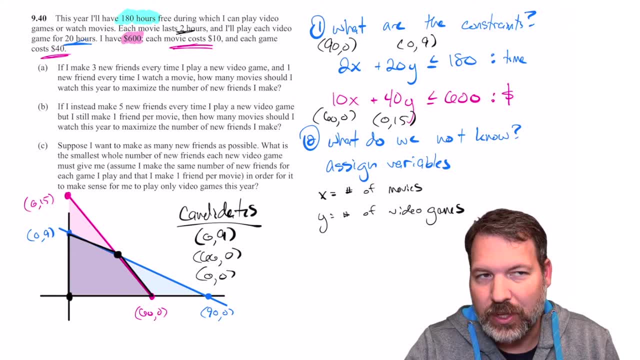 typically the origin, and if we're maximizing something, we would almost always presume it's not going to be maximized at the point where we do nothing, In this case, watch no movies, play no video games. But just for completion's sake, we're going to include 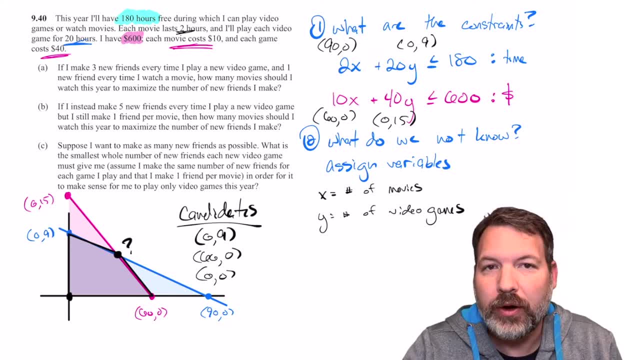 that maximizing point at the bottom left-hand corner, And so we've got 0,9.. And so we've got 0,0.. The only other corner we don't know about right now is the intersection between our two boundaries, And there are several ways to figure out what that intersection is. One thing you could: 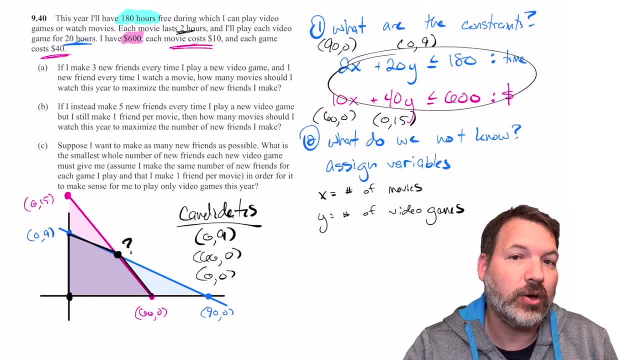 do is take your linear inequalities, treat them like linear equations and then solve that as a system of equations, Whatever the ordered pair is. that's the solution to that system. is the corner of that region, But, like I said, I actually want to have a graphing calculator. do? 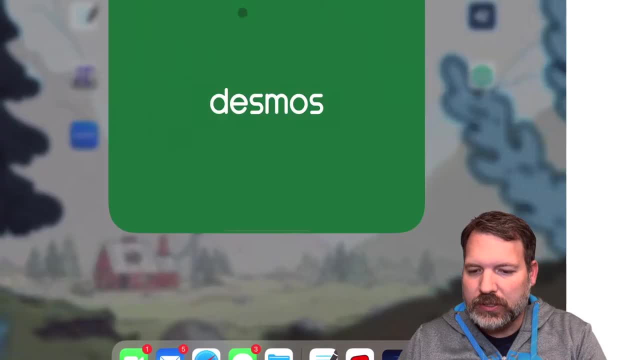 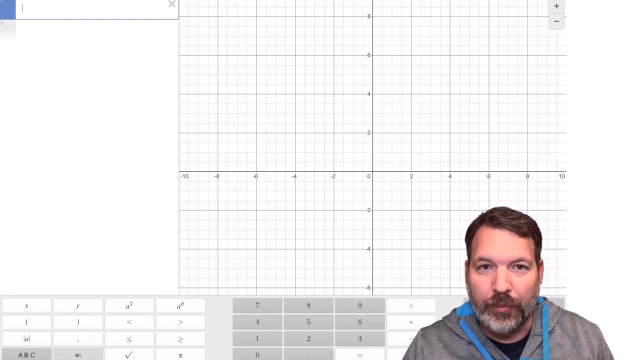 this for us. I don't want to do this by hand, So I think it's time Let's go And open up Desmos. We're going to graph this system And we're going to figure out what the possible solutions are for the thing that we're maximizing- Which, by the way, we haven't even. 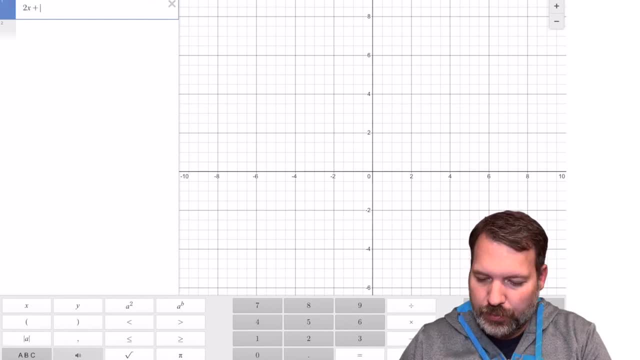 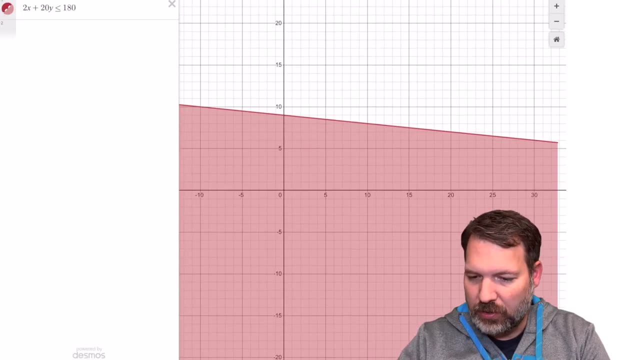 looked at yet the actual question, But we'll get there 2x plus 20y, less than or equal to 180.. So we're going to have to zoom out a little bit, figure out a good window for this. There we go. 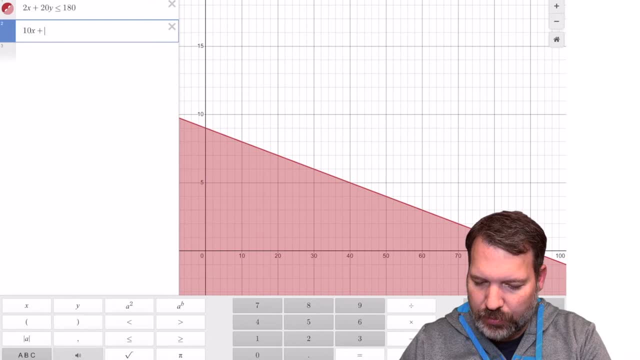 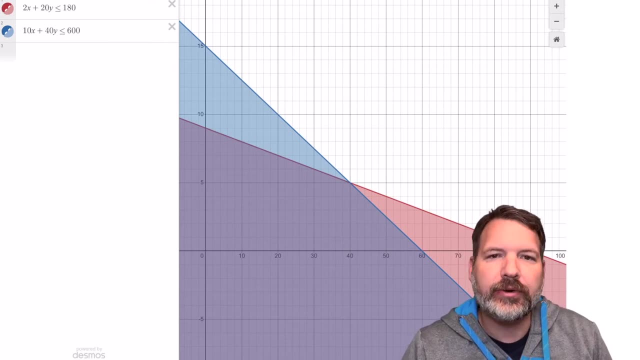 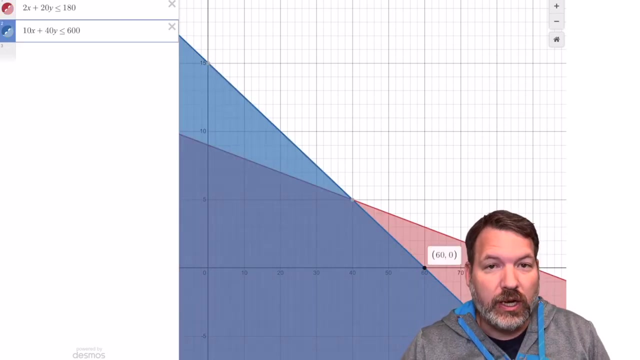 That's looking pretty good. And then the other one was 10x plus 40y less than or equal to the $600 that we have to spend, And that's pretty good. Our sketch roughly looks like what's going on here right now. We've got some points like 0, 9.. We saw that one: 60, 0.. And then the one we 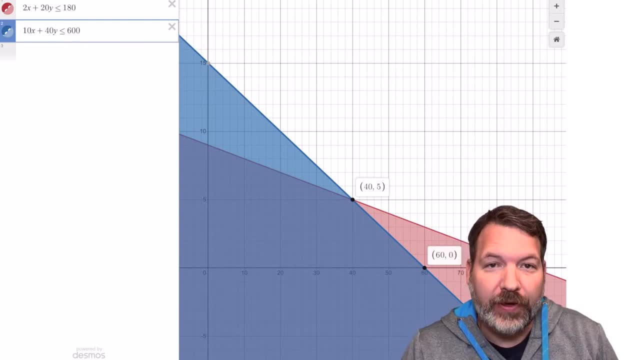 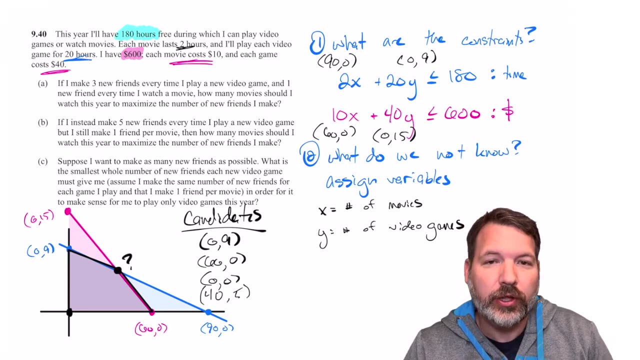 didn't know about the intersection point 40, 5.. Let's just record that so we remember that for the future: 40, 5.. Now, like I said, we actually didn't even look at the actual question. Let's go. 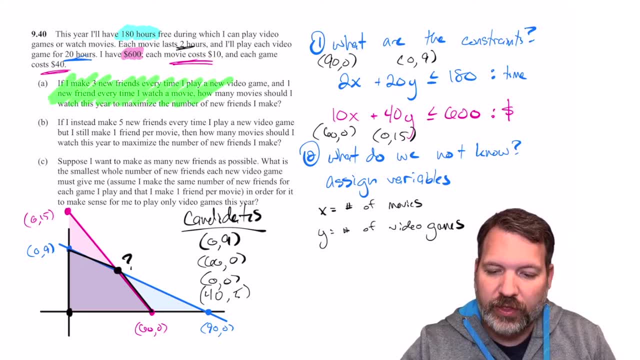 ahead and jump into the actual question here. There are in fact three of them, But we're going to talk about the other one, So let's check out the other one. If I make three new friends every time I play a new video game and one new friend every time I watch a movie, how many? 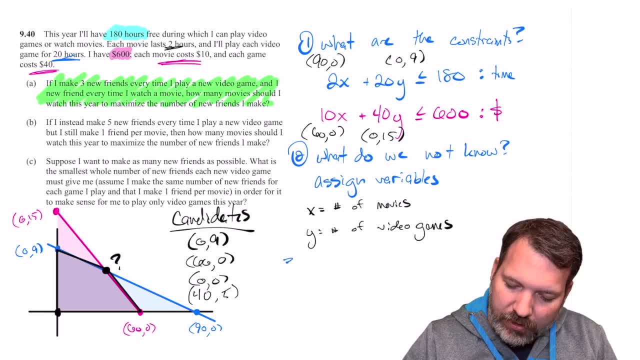 movies should I watch this year to maximize the number of new friends that I make? So we are maximizing our quantity here. Now. this is our step three. What is our objective? What is it that we're actually trying to optimize? to make as large or as small as possible? Again, in this case, it's 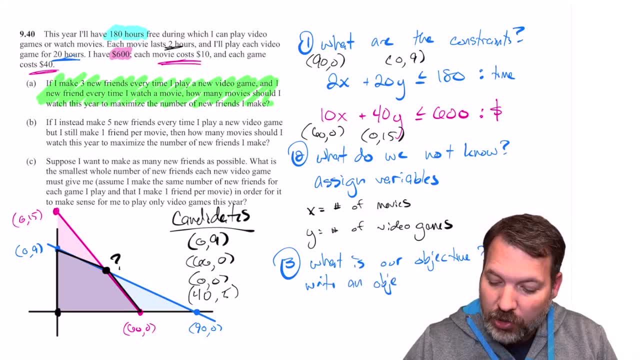 friends And we're going to do the same thing. We're going to do the same thing, but we're going to to write an objective equation, Again objective, related to goal. In this case, our number of friends, which we will call F, is coming from one friend per movie. 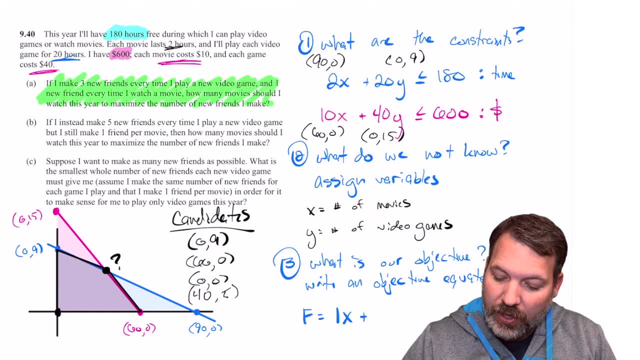 so that's one times the X number of movies we watched this year, plus three per video game. so that's plus three times Y. All we need to do now is take these four candidates, these four corners- these are the only possible optimizing points- plug them into this equation. 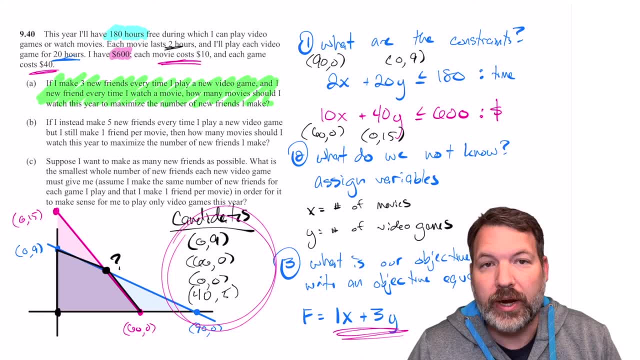 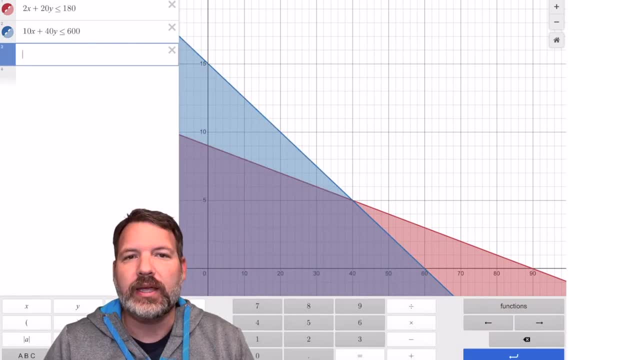 and whichever one gives us back the most number of friends the greatest number is the answer to at least part A of this problem. But let's go ahead and justify that I said I would show you why it is that the corners are always going to be your maximizing or minimizing points. 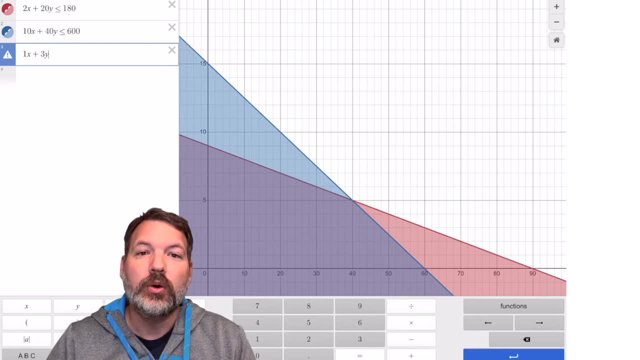 So we have this equation, one X plus three Y, which itself is a linear equation. If you put something like equal to zero, that green line down there in the bottom left corner is what it would look like. If you put equal to 10, it would kind of slowly move. 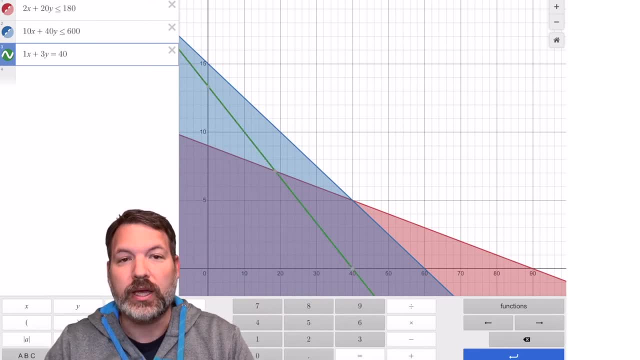 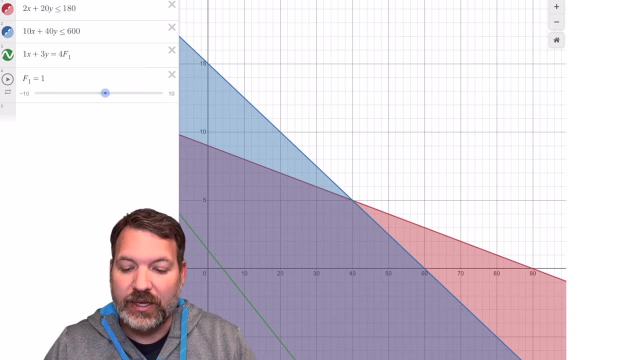 to the right. equal to 20,, equal to 30,, equal to 40, that line is moving to the right. If we just say in general, it's equal to something we're gonna call F1, Desmos, lets us add a slider. 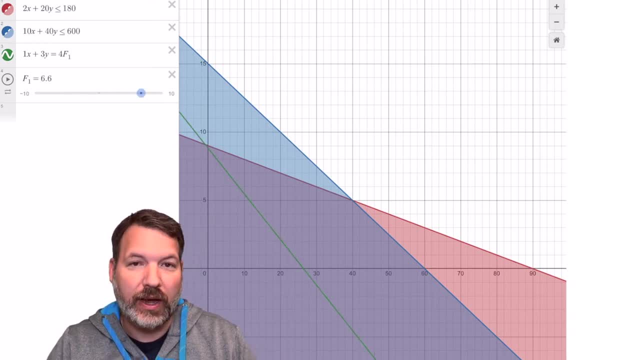 which can kind of dynamically show us what's going on with this line And as we move it across our space. remember, the space we're interested in is that kind of diamond shape. In fact, let's go ahead and get that diamond shape. 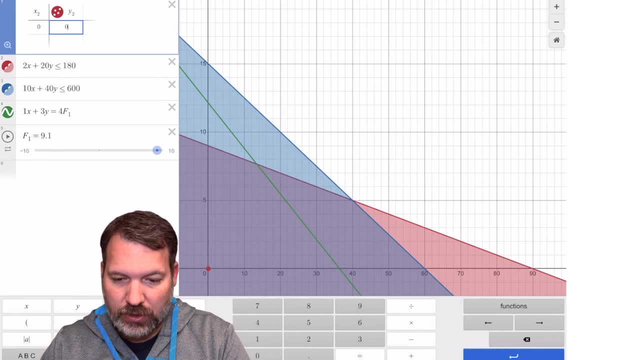 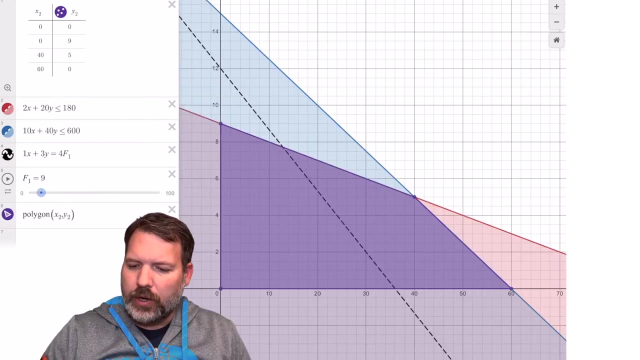 down real quick. So we had corners at zero, zero, zero nine. Where was the solution? 40 comma five, was that corner there? and then 60 comma zero. Okay, we're gonna have Desmos graph that space in there for us in purple. 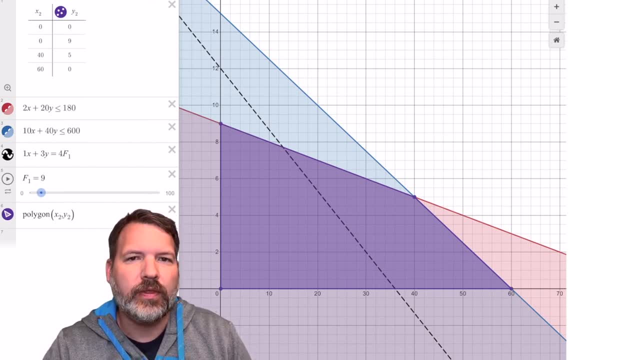 All right, there we go. So we've got that purple polygon And again that represents the shaded region under both of our linear constraints. Any ordered pair in that purple region will satisfy both of the inequalities. What we're trying to do is maximize this black dotted line. 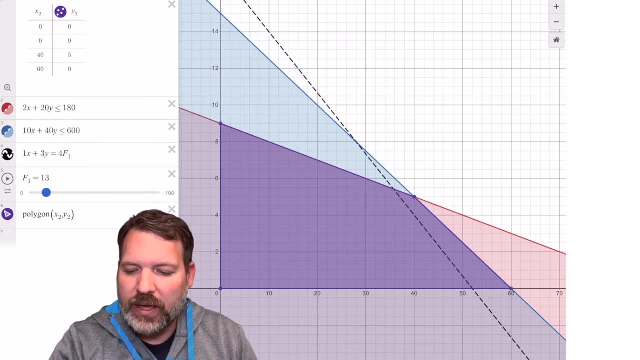 And what I'm trying to justify to you is: why is it that the corners must be the maximizing points? You can see as we move that one X plus three Y line, it can reach greater or lower values. That's what the slider is showing us. 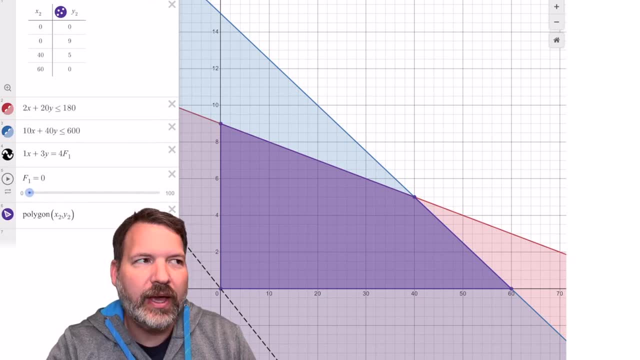 But when it reaches a least possible value, it's going to have to be intersecting our region at just one single point, just the one corner. As we move it across the region, at some point it will reach some point. It will reach some other of the three corners. 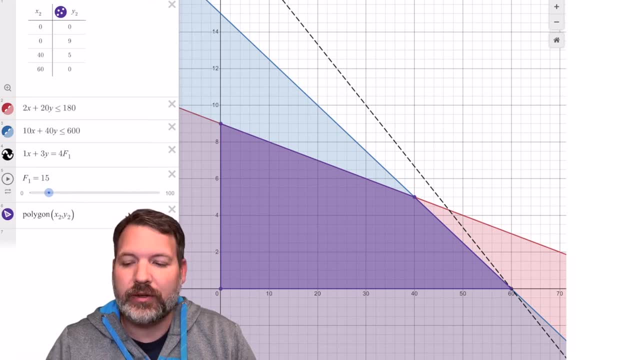 and that's where it's reaching a maximum value. So you can actually already tell here the dotted line is giving us the information that that bottom right-hand corner, 60 comma zero is maximizing something, In this case maximizing our number of friends. 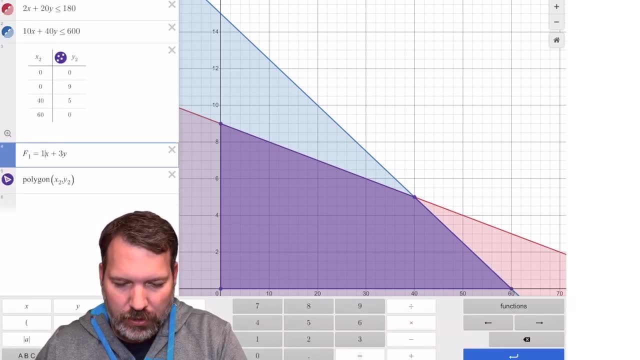 In fact, as long as we're having Desmos do this for us, let's just have Desmos compute it as well. Let's see, this is X two, that's Y two. We've got F one being the possible amounts of friends. 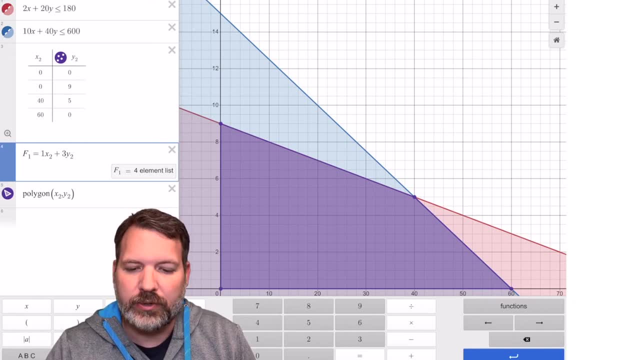 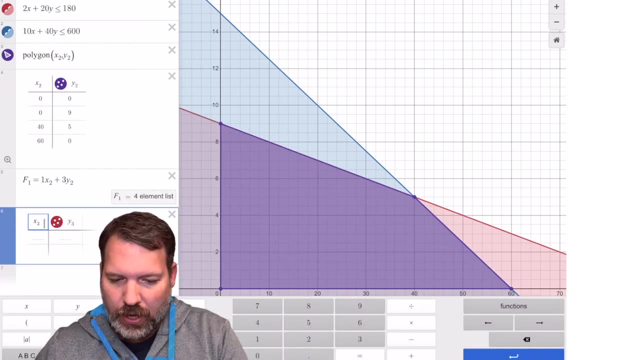 given these different ordered pairs- zero comma zero, zero comma nine and so on. We're actually going to go ahead and build another little table here And on the left side of the table. we just want four different entries for the four different possibilities. 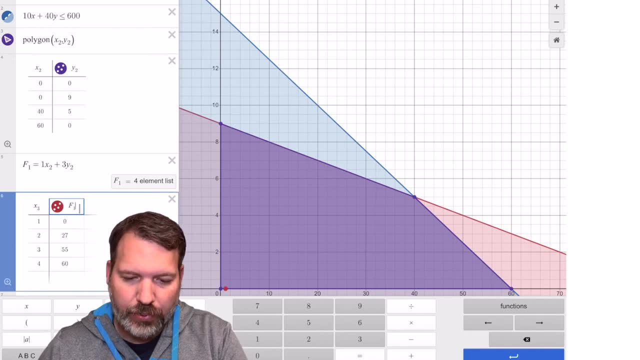 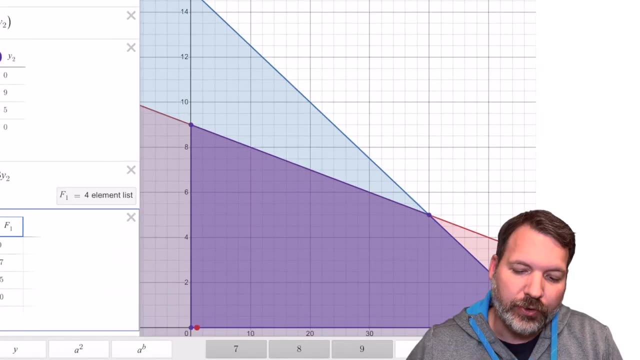 that we're checking out, And on the right side of the table we want it to compute F one for us. and there it is. Those are the four different possibilities for the number of friends here. So, for example, this first entry in our list. 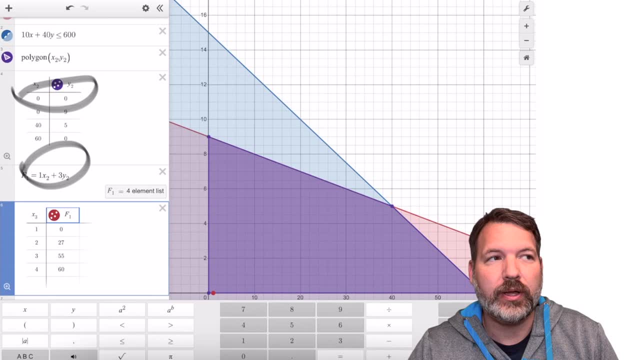 zero comma zero. Well, if I multiply that first zero by one and that second zero by three, I make no friends at all this year. Obviously that's not gonna maximize anything. but that's what we said about the origin. It's probably not going to maximize for us. 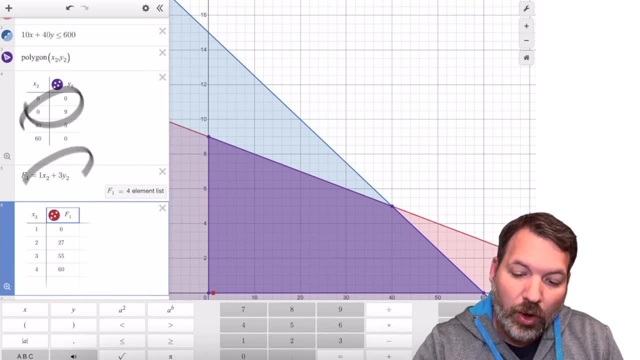 On the other hand, if I plug in this second point, zero comma nine. one times zero plus three times nine makes 27, and that's what the second row in that second table is telling us Clearly. what we're interested in is where that second column F one. 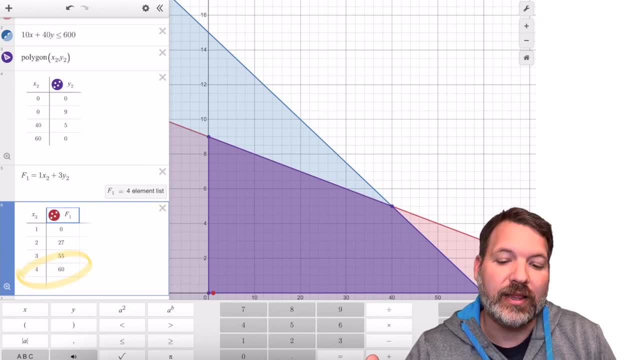 our number of friends reaches a maximum, and in this case, that is at the fourth point, 60 comma zero. If I make three new friends every time I play a video game, one new friend every time I'm watching a movie. 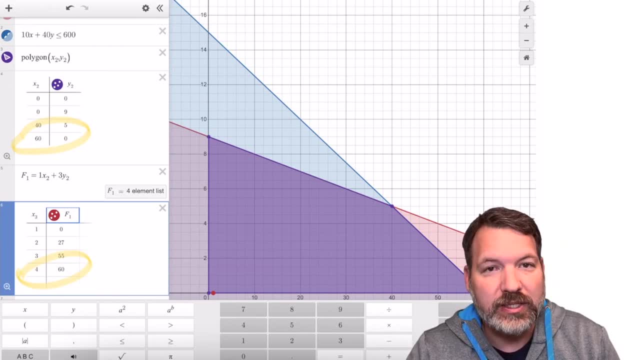 and given the other constraints here- the money and the time that I can spend on movies and video games- then the best thing to do is actually just to watch 60 movies this year and therefore make 60 friends. So that could be our answer to part A. 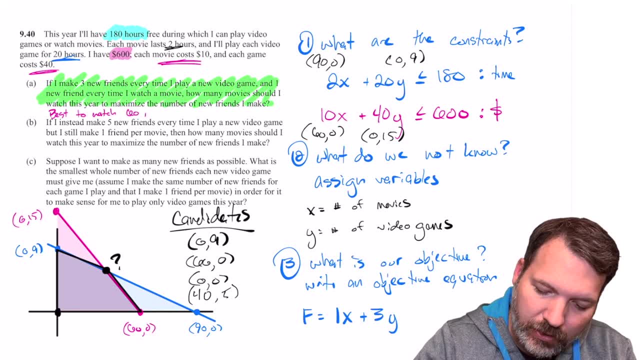 It's best to watch 60 movies. I have the money to watch 60 movies, I have the time to watch 60 movies, and so I'm going to make my 60 friends by watching 60 movies. So that's it. 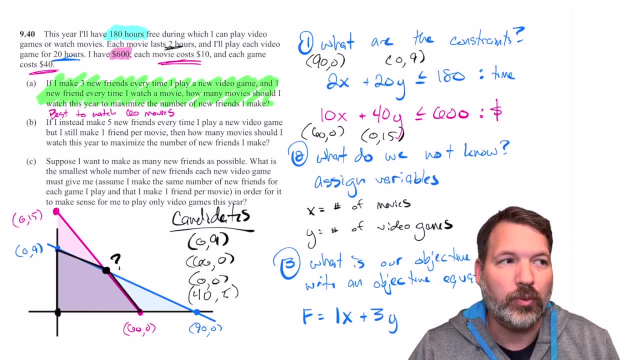 That's linear programming. That is a traditional linear programming question where we have our objective. The weights for the objective are given to us. That is, the one friend per movie, the three friends per video game. We take the corners from those two linear inequalities. 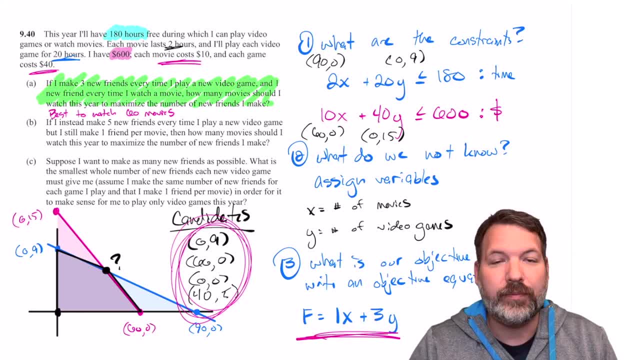 that we graph, plug them into the objective equation and then pick the either maximizing or minimizing point, Which, again in this case, happened to be this bottom right hand corner, 60 comma zero. Just to finish it out, though, this particular problem asks us to go on. 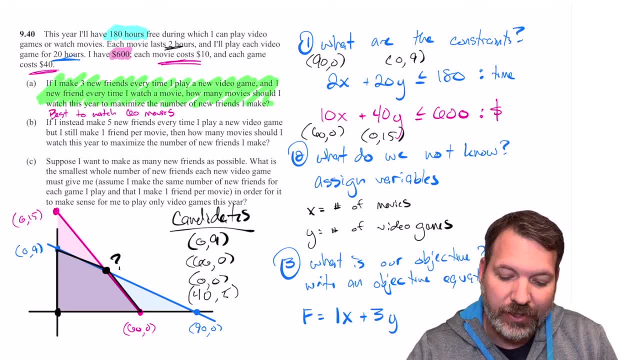 Part B gives us a different scenario to consider. Part B says: suppose that actually we make five new friends every time we play a video game. So one thing you might've noticed earlier on in the problem is, in a sense we get more bang for our buck. 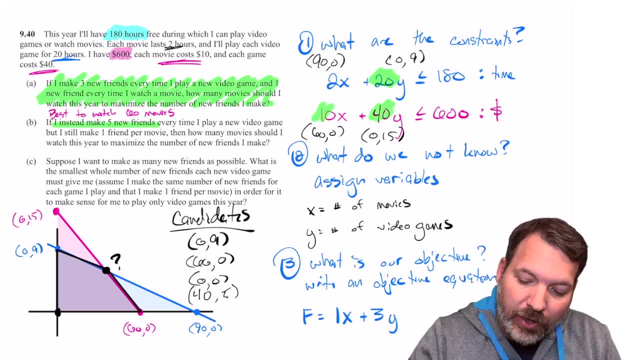 out of the video games. They cost four times as much as the movies do, but we get 10 times as many hours of play out of the video game than we do from the movie. In one sense, that means that video games are actually very resource intensive. 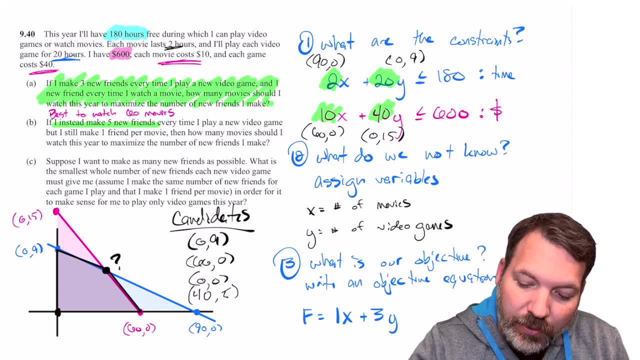 They cost more and they take more time, But if what we ended up seeing is that they also helped us make more friends- I mean, they already were before. three obviously is bigger than one, but it was only a times three advantage. If, instead, video games actually helped me. 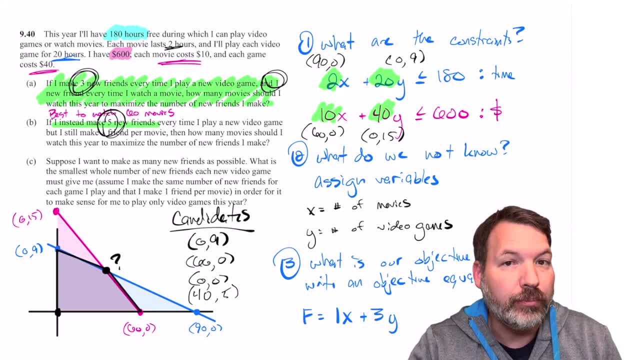 make five new friends compared to the one new friend for the movies, then I might see this relationship change. Now this is gonna require that I adjust my objective equation. In fact, here I would now say that F my number of friends. 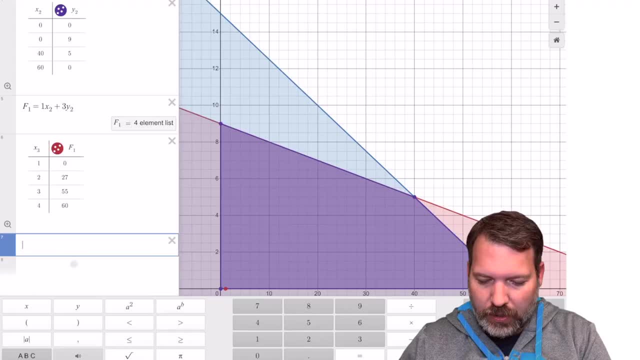 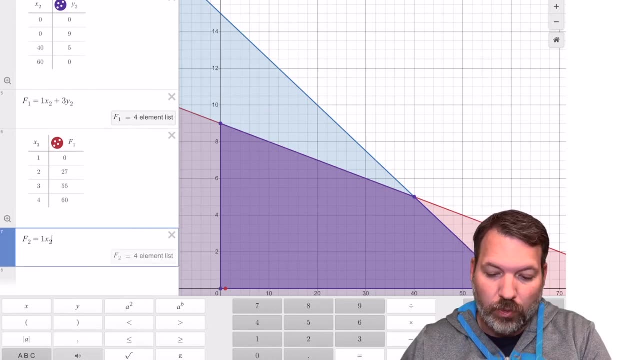 is equal to one times X plus five times Y. Again, I don't wanna have to do this math myself, so I'm gonna have Desmos do it, computing something I'm gonna call F2.. F2 equals one times the number of movies. 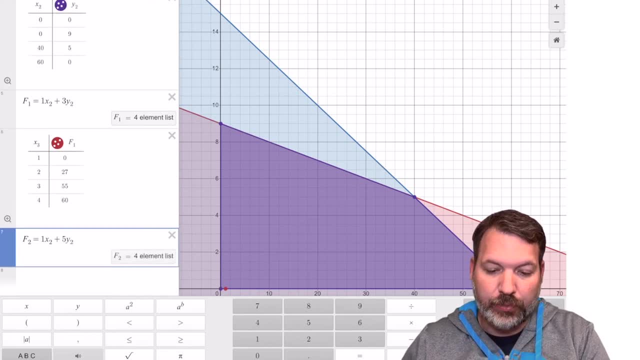 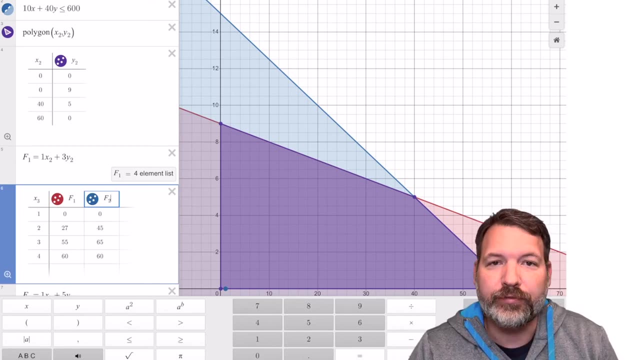 that I watched this year, plus five times the number of friends. Can I get it onto the same table? Oh, very good, I can, And so now I have some new values for the number of friends I end up with at the end of this process. 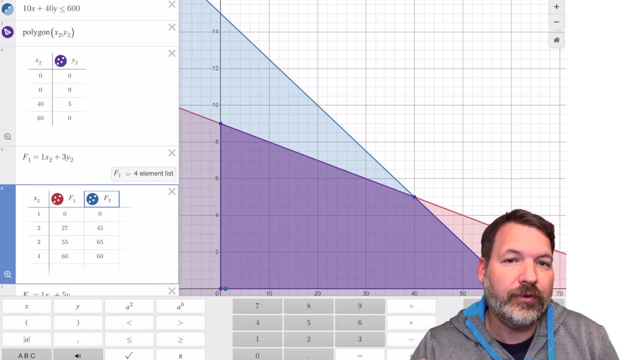 at least in some of the cases. You'll notice that the first and fourth points here, that is the origin, and then that bottom right-hand corner, 60 comma zero. in those two cases the number of friends remains the same. I'm still making zero friends at zero comma zero. 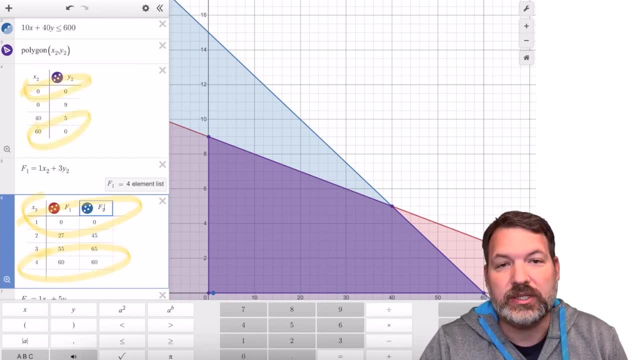 I'm still making 60 friends at 60 comma zero. But what is changing are these other two values, because those values had non-zero numbers for the number of video games that I'm purchasing, And what we changed in our objective equation was how many friends I make per video game. 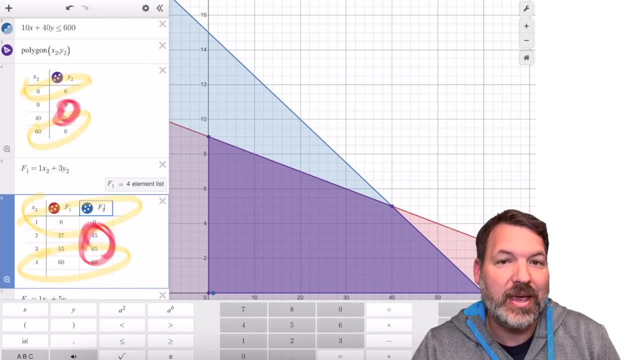 Since it's five now rather than three, I can see I'm making more friends at those points. In fact, it happens to be just enough that it is now worth playing some of the video games If I spend my time and money on 40 movies this year. 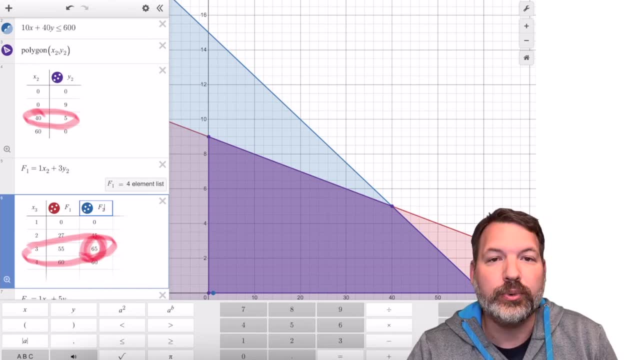 but five video games, I'm gonna end up with 60 friends. I actually maximize my number of friends at 65.. That's coming again from: one times 40 is 40, plus now five. I've changed the weight. five times five makes 25, and 40 plus 25 is 65.. 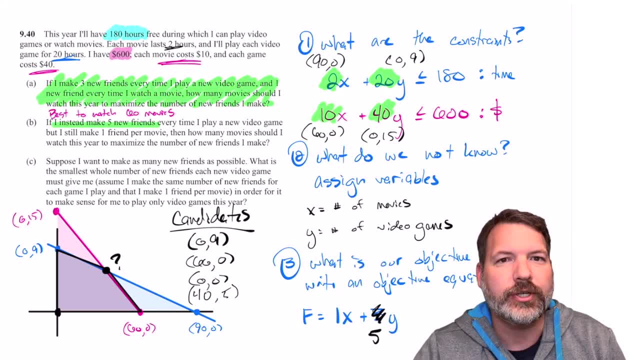 One last little question here, part C, very weird question, unless you're using something fantastic like the Desmos graphing calculator, Suppose I want to make as many new friends as possible, What is the smallest whole number of new friends each new video game must give me? 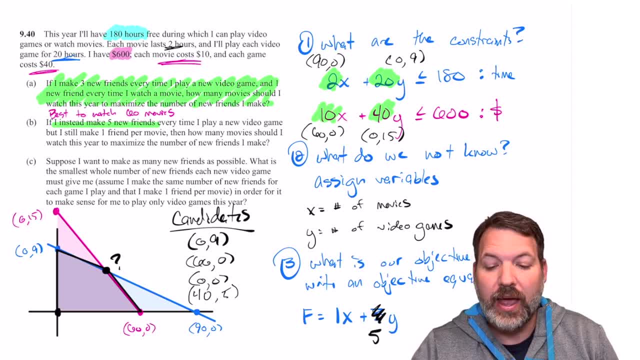 Assume I make the same number of new friends for each game I play and that I make one friend per movie. So we're basically holding the one friend per movie constant, but now instead of necessarily three friends per video game or even five friends per video game. 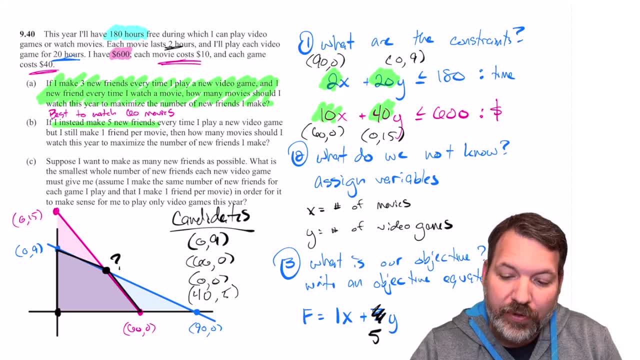 I get to pick that number, I get to choose the weight. What would be the first whole number of friends per video game where it would actually make sense to only spend time and money on video games? Like I said, Desmos makes this pretty easy. 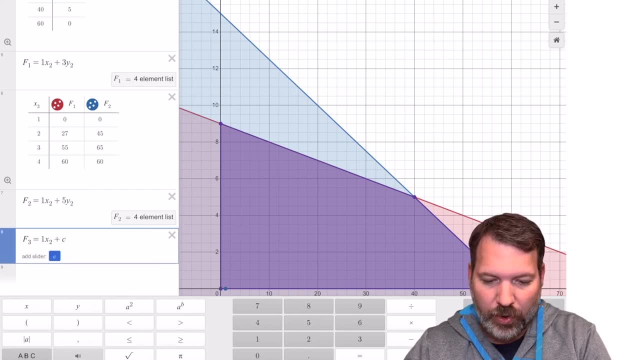 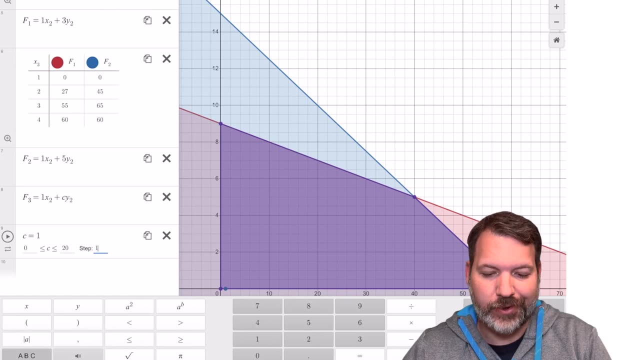 to do? we're just gonna write this equation here. We're gonna change the weight- not three, not five, but C. We're gonna have Desmos. add a slider. They said it had to be a whole number, so let's assume it's gonna happen somewhere. 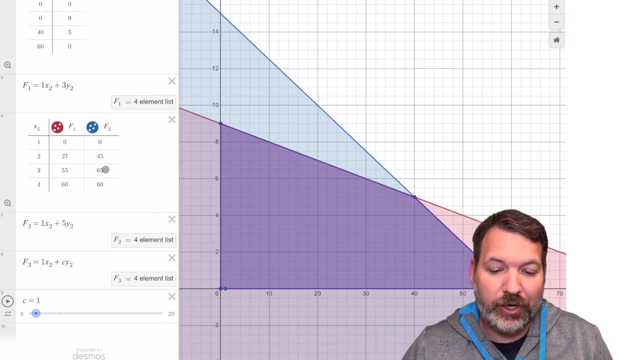 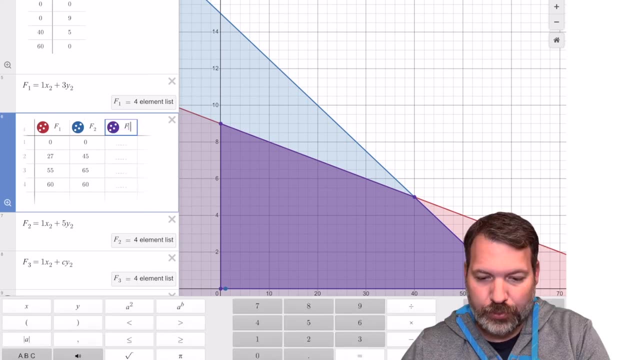 between zero and 20 friends per person. And again, we actually already know that, when we move from three friends per video game to five, that the video games are starting to look more attractive to us. Put in one more row here for F3,. 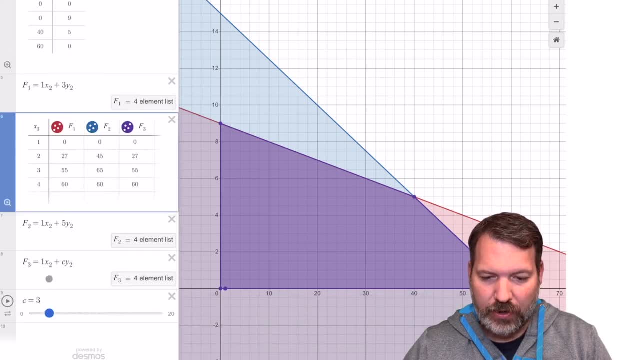 and all I'm gonna do is kind of adjust this slider And what you can see happening again, those middle two boxes are the ones that are changing because as we're increasing this weight, we're making video games more and more popular. We wanna know the first number. 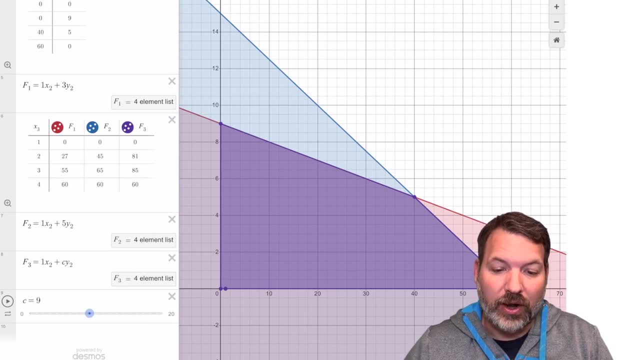 where we can do only video games. You'll remember that only video games was the second level. so I'm looking at this second row And right now at C equals nine, that is, nine friends per video game. it's not quite better. 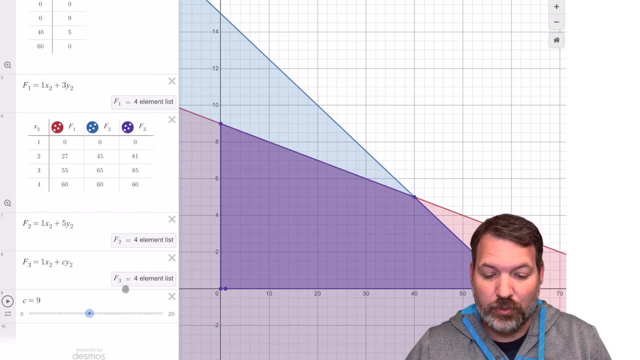 It's still worth spending some time on movies. That's what I'm seeing in row three. If I bump it up to 10,, however, you can see that these two rows are now equal And finally, at C equals 11, it's actually better for me. 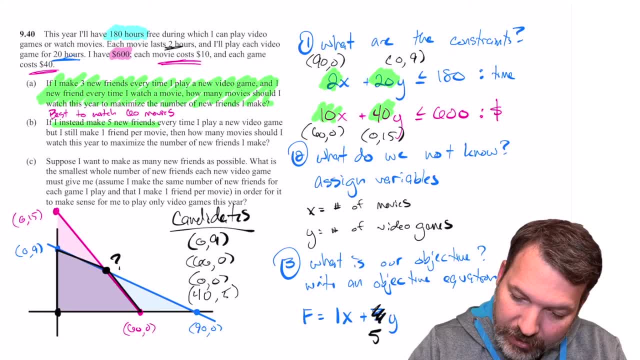 if I just spend all my time on video games now, I promise this imaginary scenario is gonna be the only time where it's best to spend all your time on video games. But the answer there make the weight: 11 friends per video game. 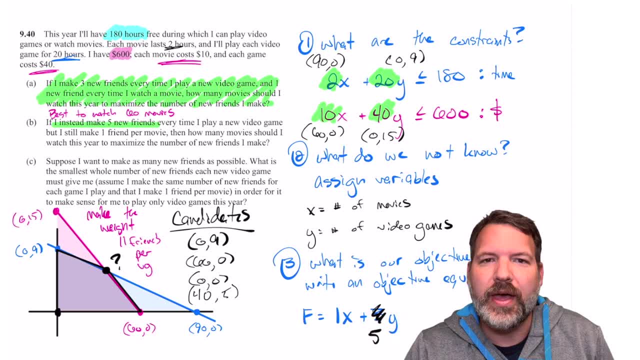 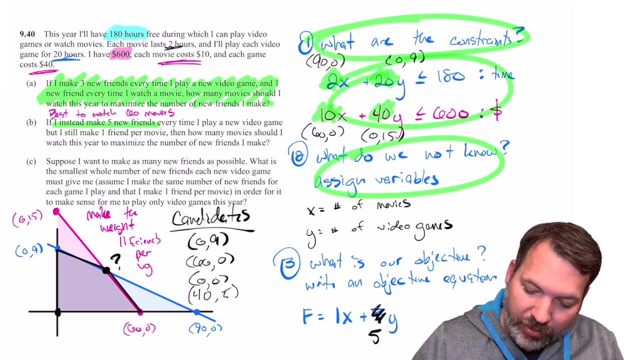 something like that Long process. Okay, but that is how I would approach this question. That is how I would approach linear programming questions in general. Again, really focus on these three questions: What are our constraints? We're going to use that along with the variables we assign. 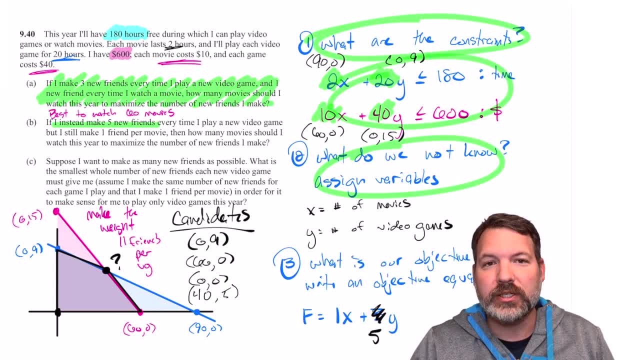 to build the linear inequalities. The solution to our system, the solution to whatever the optimization problem is, has to come from the corners. once we graph those linear inequalities, and the way we figure out which corner is best is we write an objective equation and we just plug those numbers in. 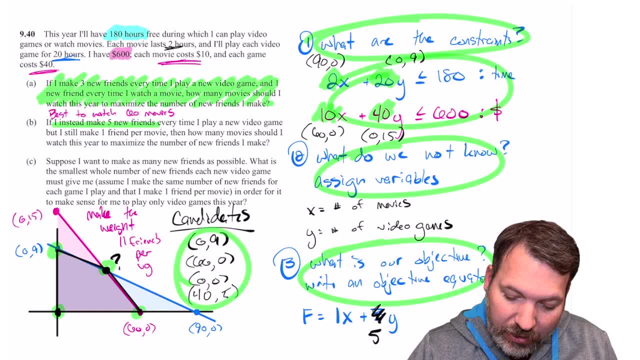 In this case I got Desmos to do a lot of the math for us but you can tell it's not terribly difficult to just plug in zero comma nine, multiply by one and three, or one and five, whatever the weights are, add it all together and look for. 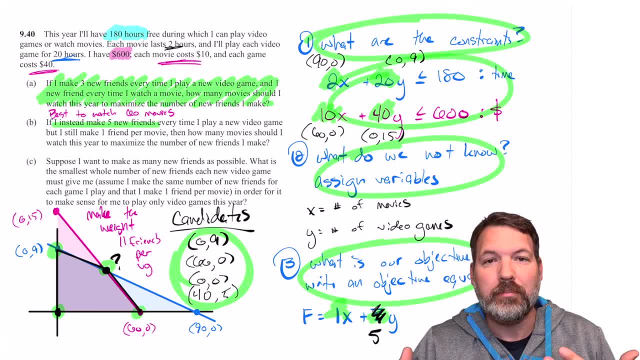 in this case, what got us the most friends. In the future, you might minimize something instead. There are lots of possible objectives, but that's the basic outline of the process. I hope that has been helpful for you. If so, like subscribe and hit the bell button. I'll see you in the next video. Bye. 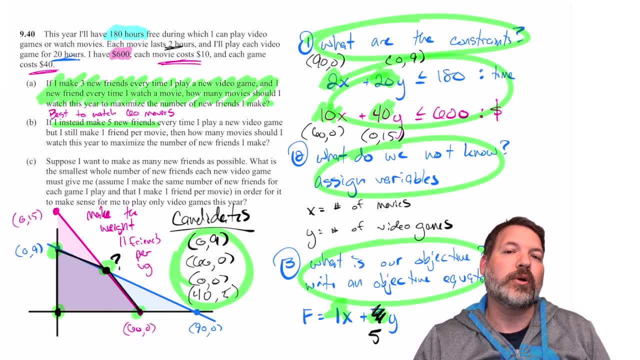 Like the video, subscribe to the channel for my students who are watching. Hey, thanks for watching all the way to the end. Hopefully this will help you on the test. I will see y'all next time. See you Please. definitely like and subscribe. 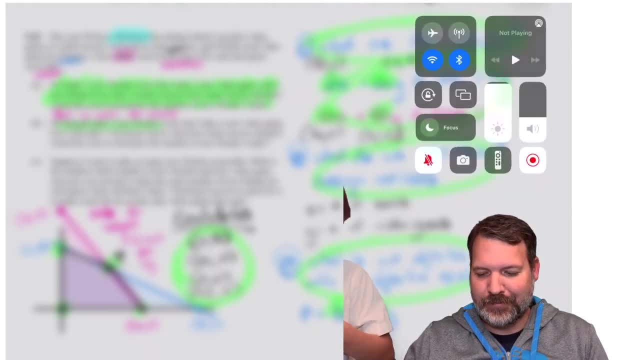 My dad's videos are super good, No.